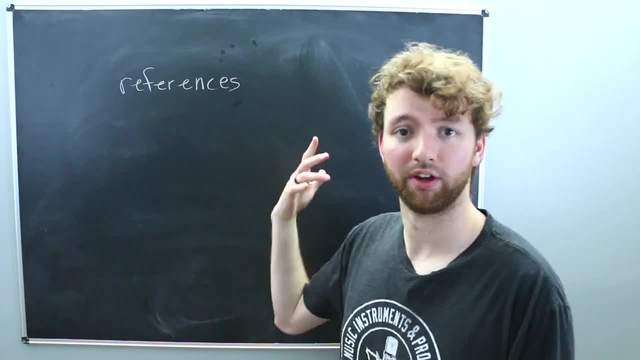 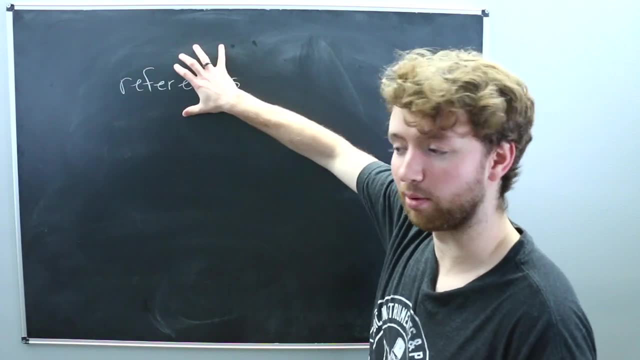 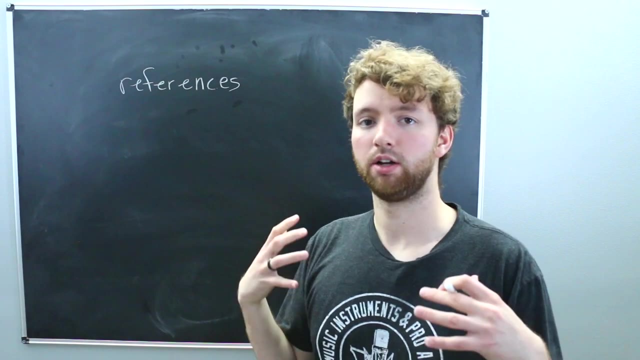 about some of the differences between references and pointers in this video and some of the upcoming content. All right, so we got that on the chalkboard: References first. Next up, let's just talk about the absolute basics: how to create a pointer, what it actually even is, why you. 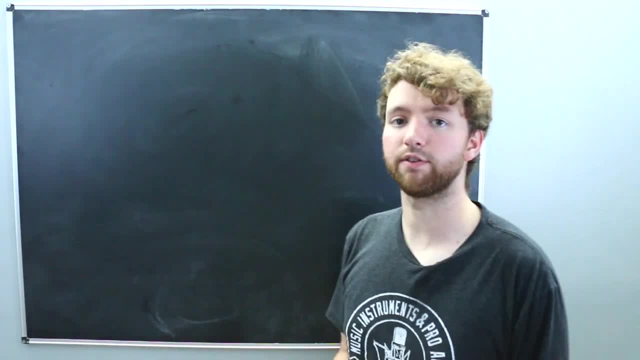 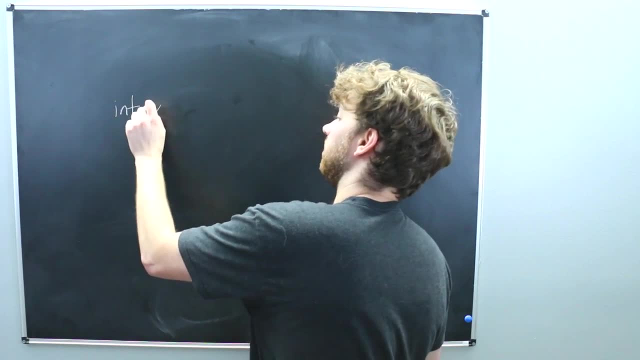 might want to use one and all of those things. So, very first thing, let's talk about creating a variable inside of C++. You say something like: let's go with, IntX has the value 5. 5.. Hey, we just created a variable, Pretty simple. You should probably know how to do. 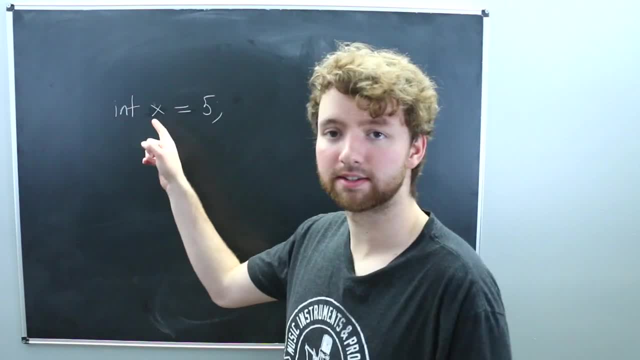 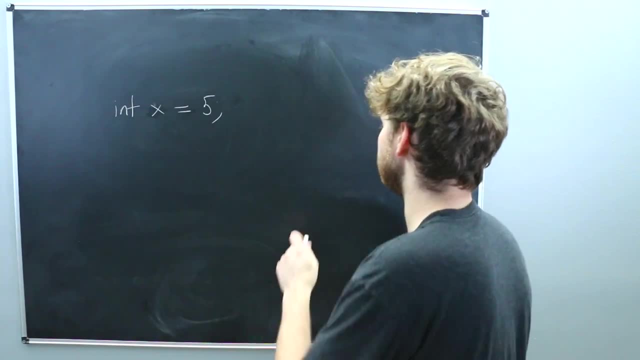 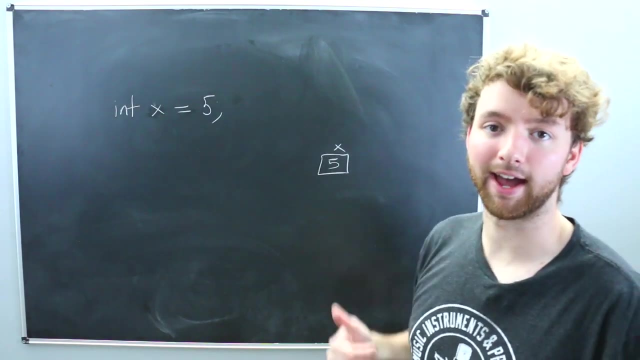 this. So right now we have this variable x, and it is of type int. So what exactly does that mean? Well, it means we have an area in memory that contains the value 5, and we can refer to it with the identifier x. But this isn't the only thing in memory. Obviously there's all kinds of variables. 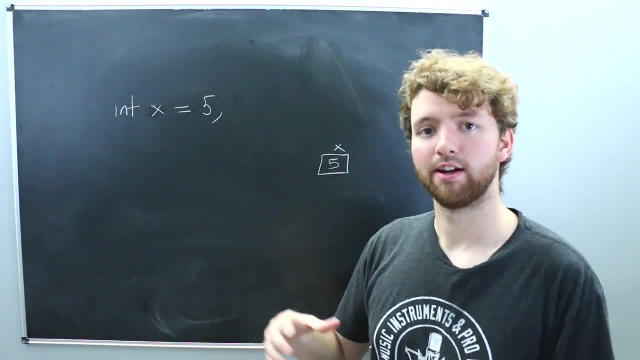 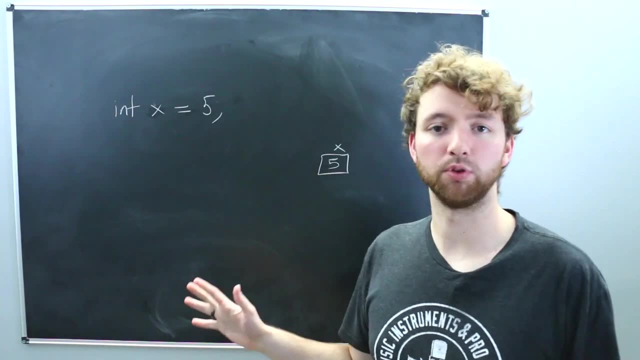 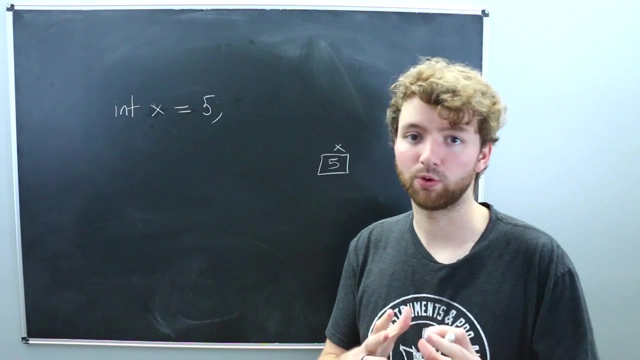 in memory and all of your programs run in memory, So you need a way to basically say where this is located in memory When you're programming. you don't have to worry about this. when you're just working with x, All that's going to happen for you. However, if you want a little bit more control, 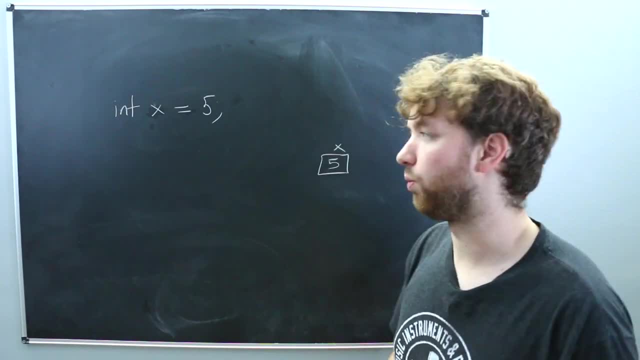 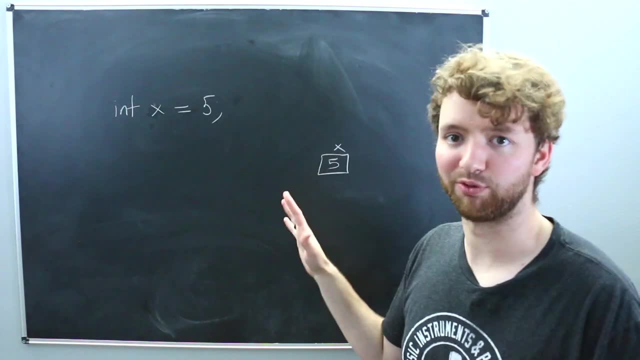 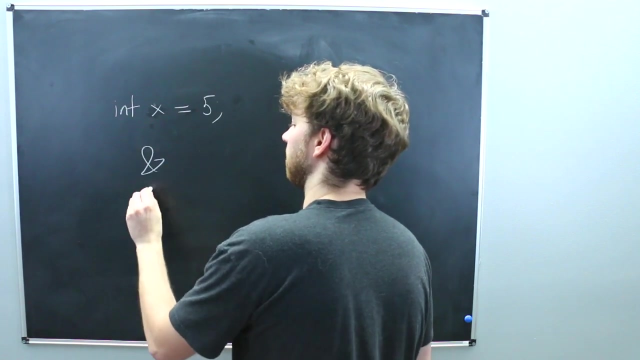 or visibility. that's where pointers come in, So we can actually point to this memory address using a pointer. All right, so before we talk about how to create the pointer, let's talk about a really useful operator, and that is the address of operator. It's kind of a weird name. 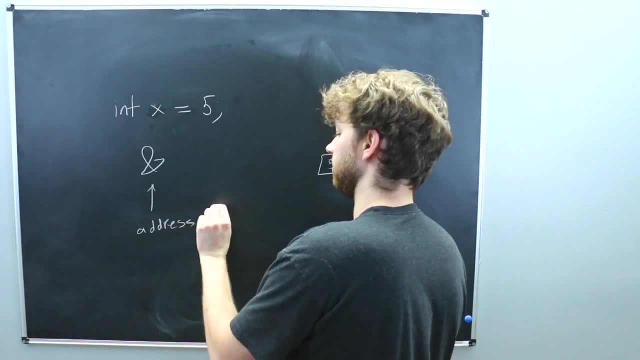 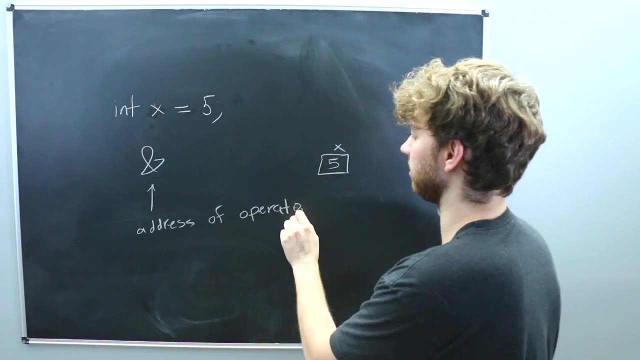 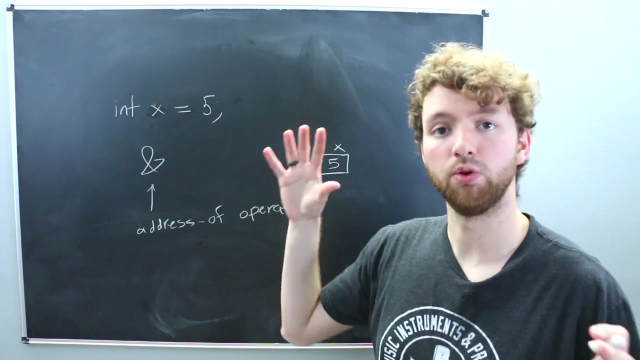 So address of operator. Dude, I don't, I can never remember if it's or or er. So this is a unary operator. What that means is it works on one operand, So you just attach it to one thing and it can be the variable. 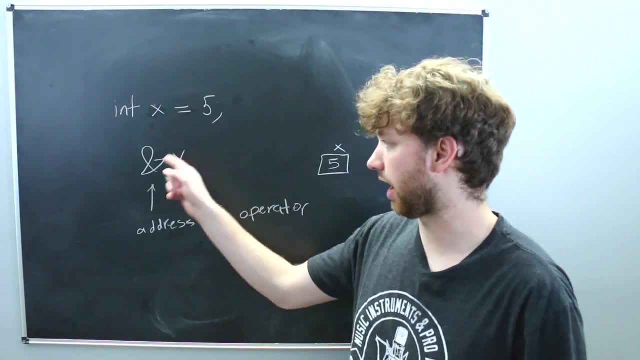 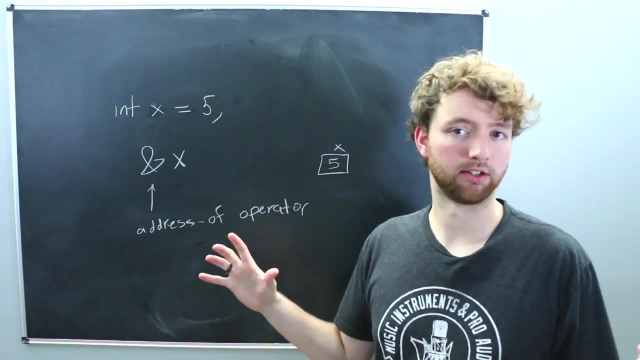 you're working with. So, basically, when you read this you you would say address of x. What does that mean? Well, it's actually going to get the memory address and it's going to probably be like 12 hexadecimal digits. I don't know why people say that, because like digits. 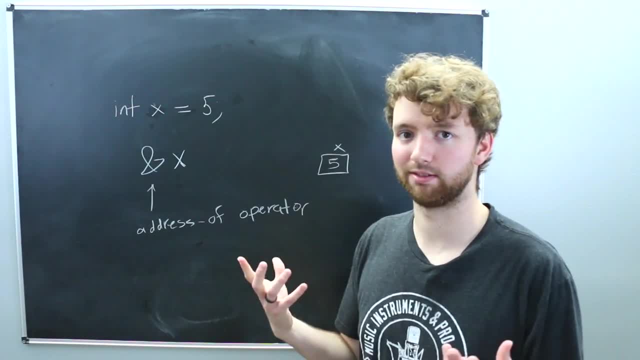 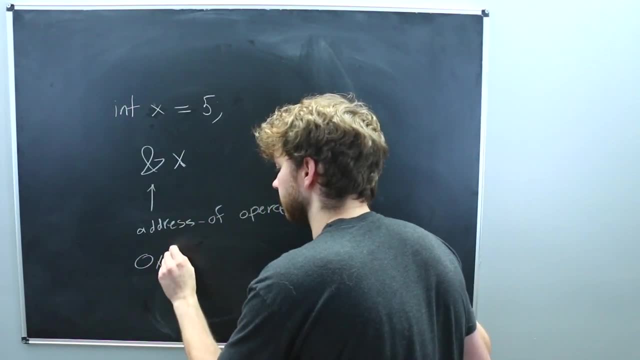 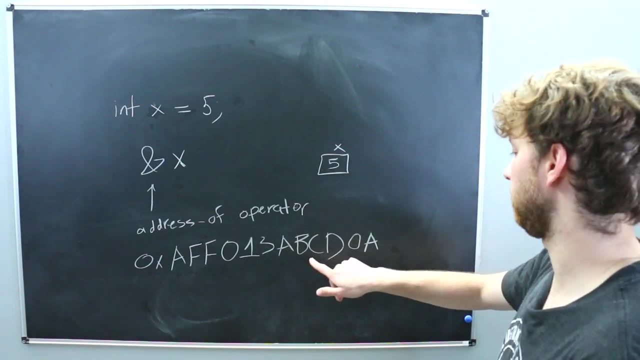 implies base 10, but hexadecimal is like base 16.. So hexadecimal numbers. So you're going to probably have 12 of those, So it might look something like this: I'm just making this up, so these numbers aren't significant, All right, so 1, 2, 3, 4, 5, 6, 7, 8, 9, 10, 11, 12.. And basically this: 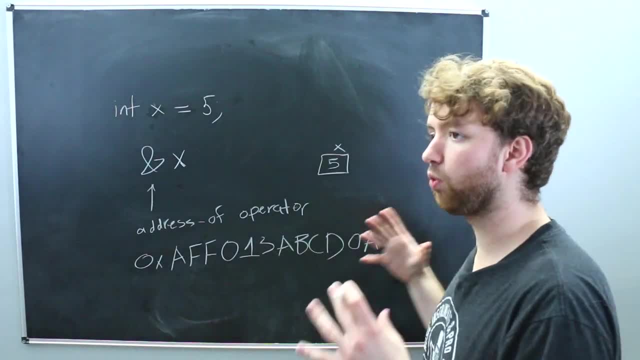 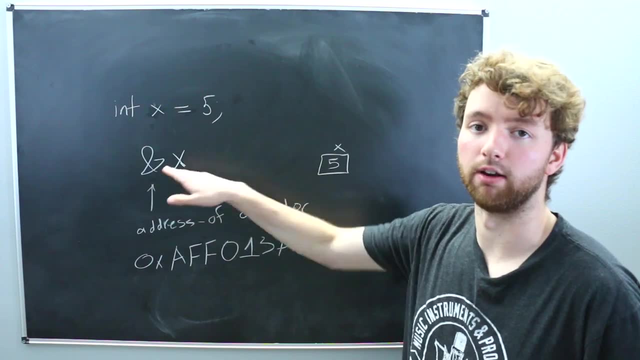 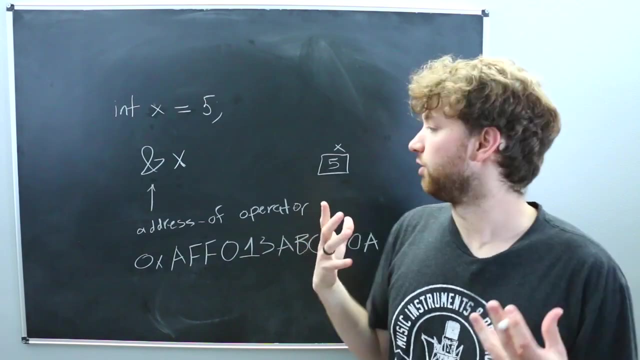 is hexadecimal, So this would coordinate to 48 bits in memory. But you don't really have to worry about that. Basically, the point is you can use this address of operator to get the location of this data right here And you don't just want to print that out. I mean you can. You could just 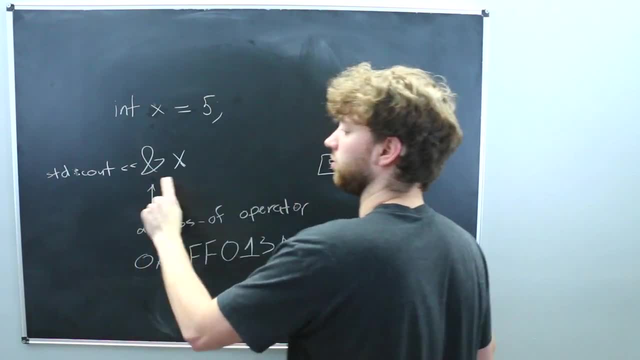 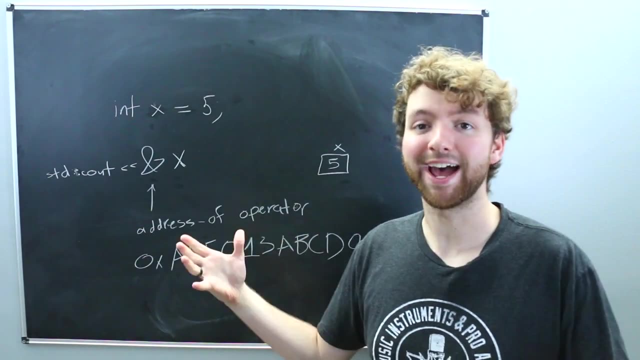 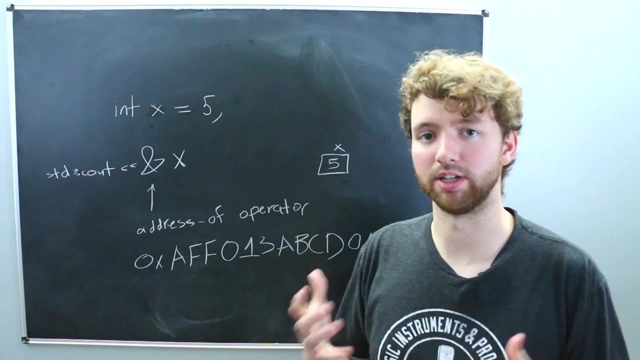 you know, say cout, like, so You can output that to the console, but you you might want to save that and use it later in your code. So I'm going to click on this and I'm going to say that bit, And, and that, my friends, is where the pointer comes in. So we can assign this to a variable and use. 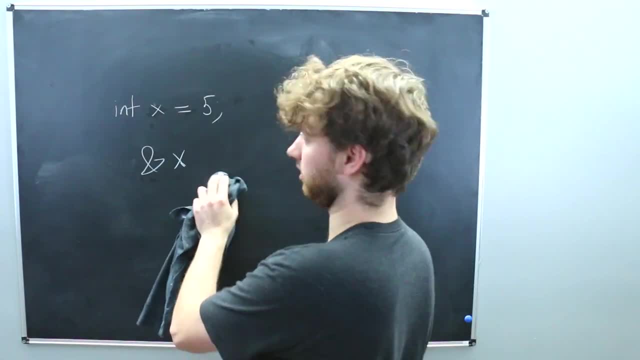 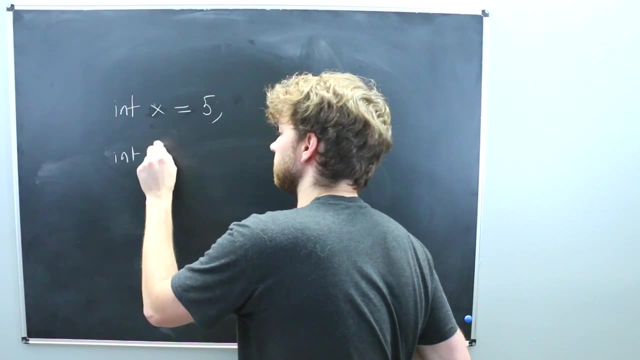 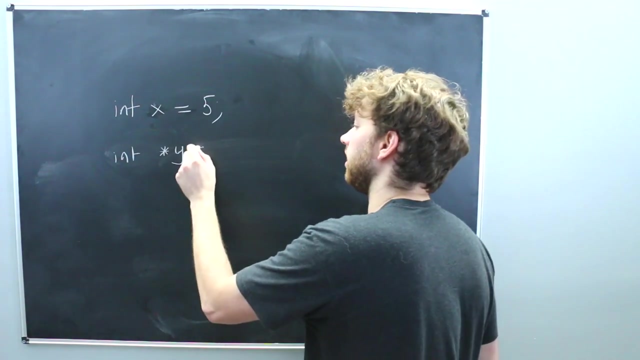 it later. So what in the world is that going to look like? Well, it's going to look like this: We're going to say int and then to say that this is a pointer, you use the asterisk and then give it a name, so, for example, y, and then you assign it the address of x, in this case. 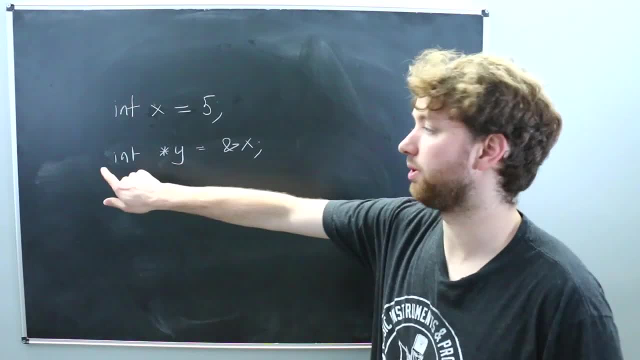 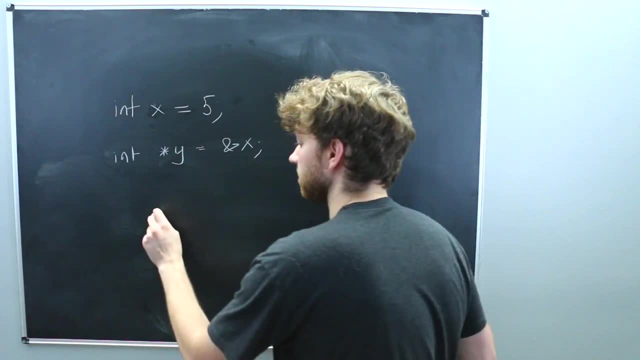 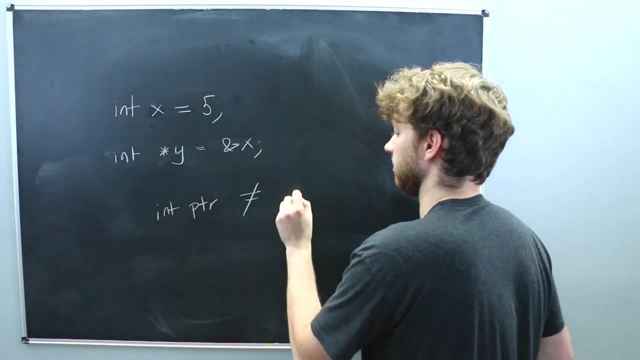 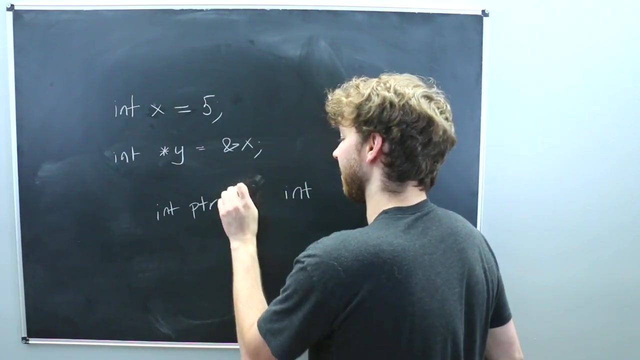 So this is the syntax to create a pointer of type int. So it's not an integer, it's an integer pointer. These are two separate types in C++. So int pointer is not the same thing as int. Sorry, I hesitated there because I'm doing like the math notation, So this is not the same. 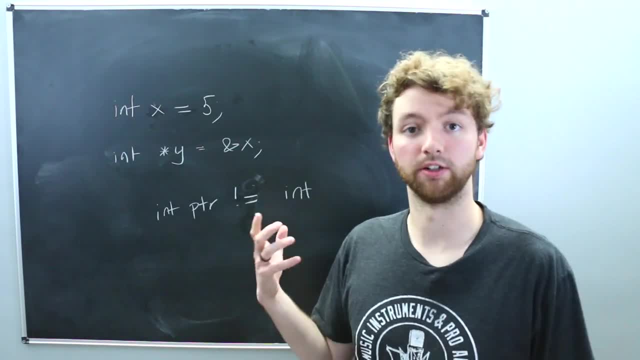 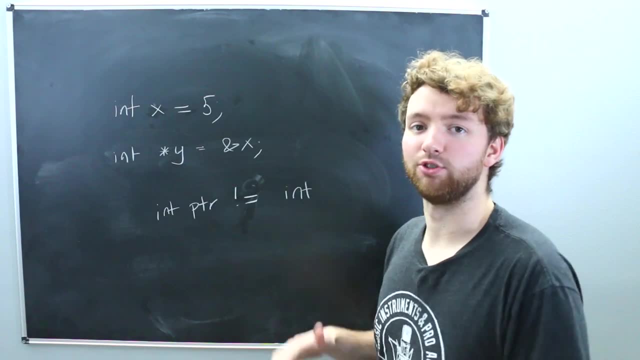 thing as an int, and if you try to use them interchangeably, you're going to get type error. things aren't going to compile or your code's just going to not work the way you would expect. So just be aware these are two separate types. When you need a pointer, you're going to use y, When 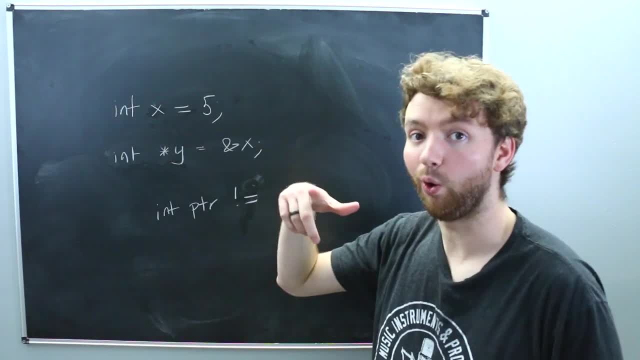 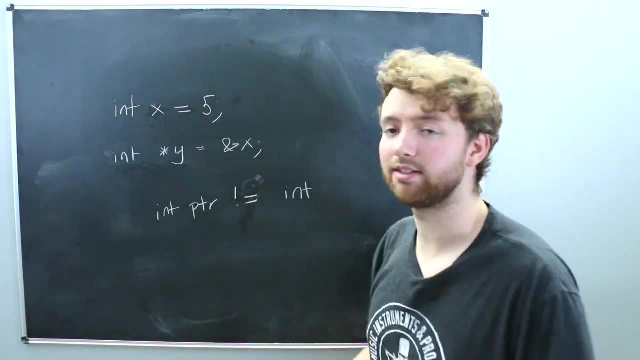 you need an integer. you will want to use x, or you can actually get the data that y points to, and that's what we're going to talk about now And again. this is kind of one of those things where it's like a lot of information, so you might need to watch this a couple times or do a little extra. 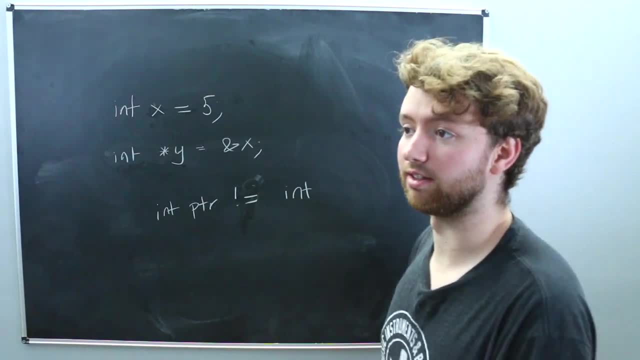 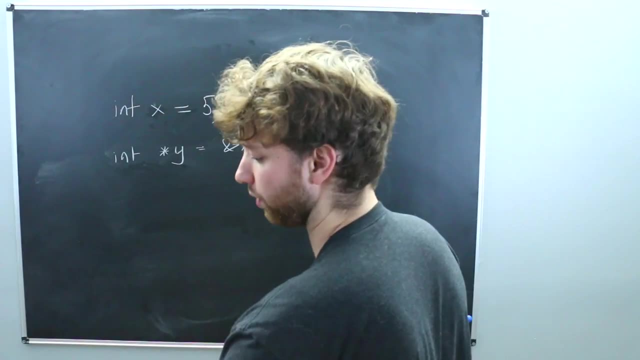 research. I'm trying to give it all in a fluid way. however, it's kind of a lot of information. It's kind of like this thing where it's like: oh, you also need to know about this and this and this, and then everything kind of pieces together, So let's just talk about what this actually looks. 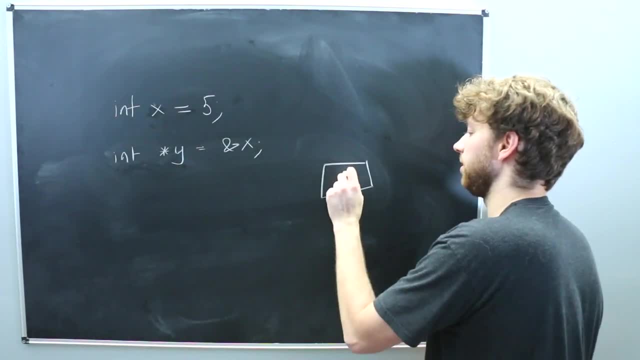 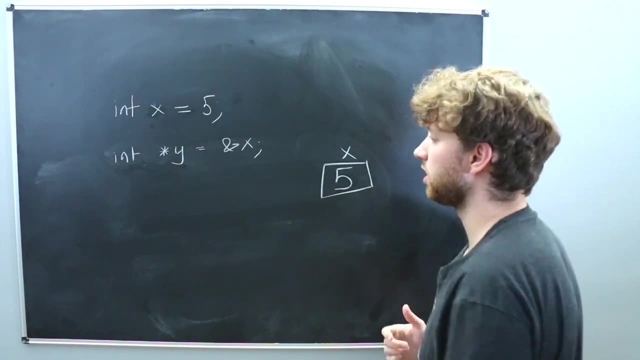 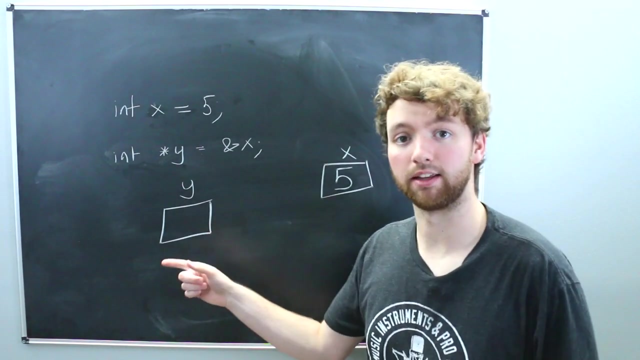 like right now. We got this place in memory and it contains the value 5 and we refer to it as x. Now we introduced this new variable and it is called y, and this is a pointer. so instead of containing the data here, it points to: 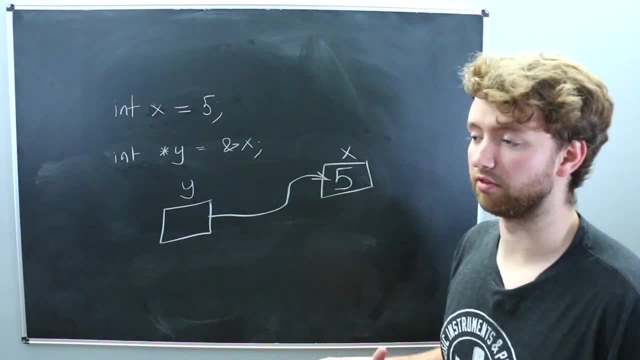 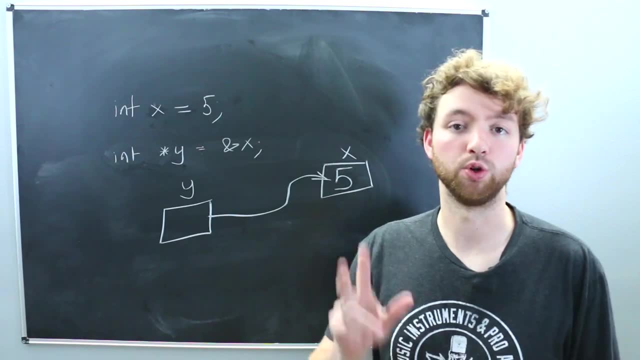 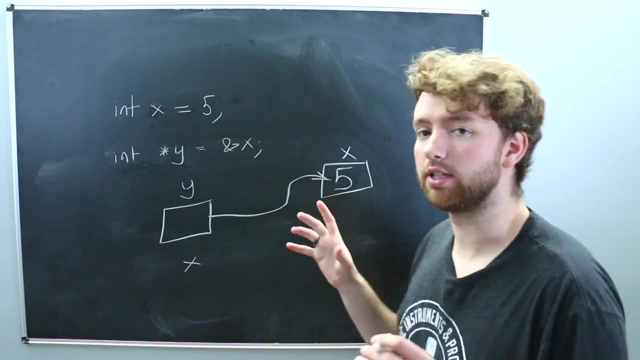 This location in memory. This is very similar to how references work, so that's why there's a lot of confusion on when to use which. So if you want to get the integer data, you can do it now two ways. You can use x, that's going to give you the value 5, or you can actually tell the computer to get. 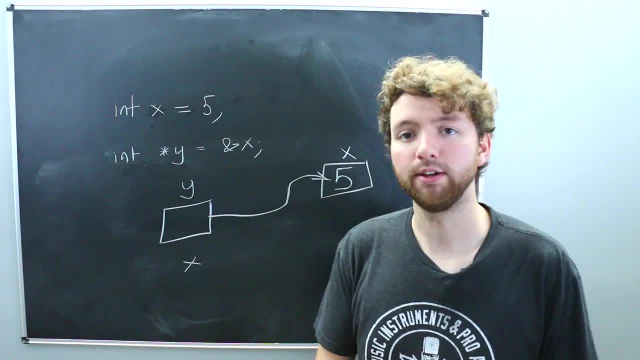 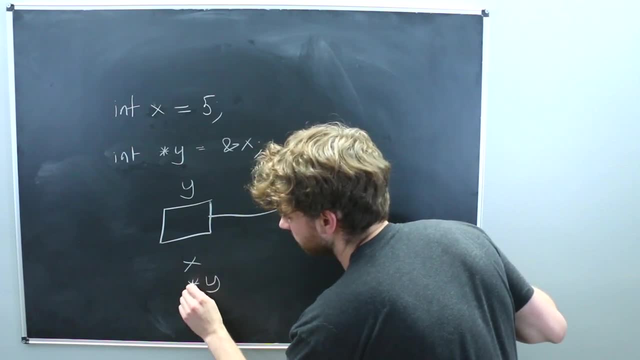 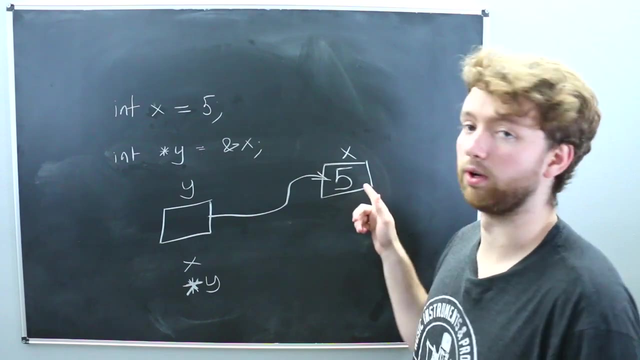 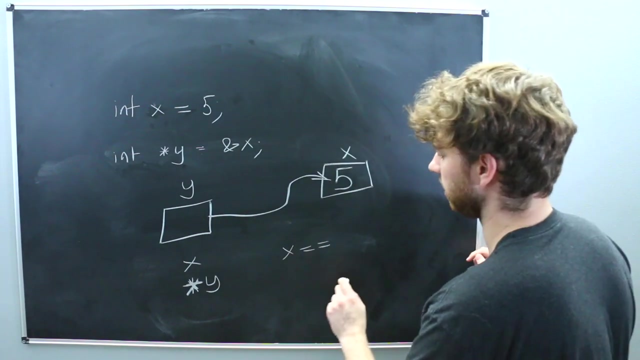 the data wherever y points, and the way you do that is with the asterisk. So you would say: asterisk y, that's a terrible asterisk- I'm so sorry guys, Something like that. So asterisk y, that is also going to give you the value 5.. So if you were to compare these, x being equal to asterisk of y, 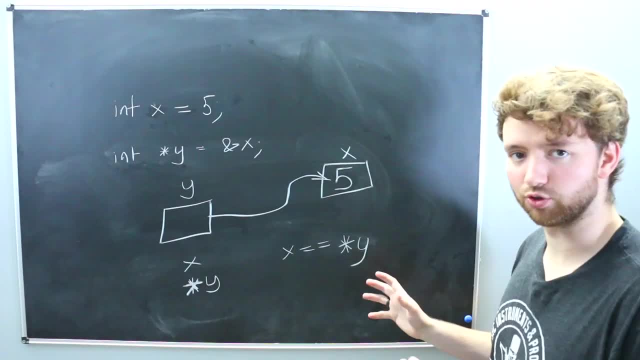 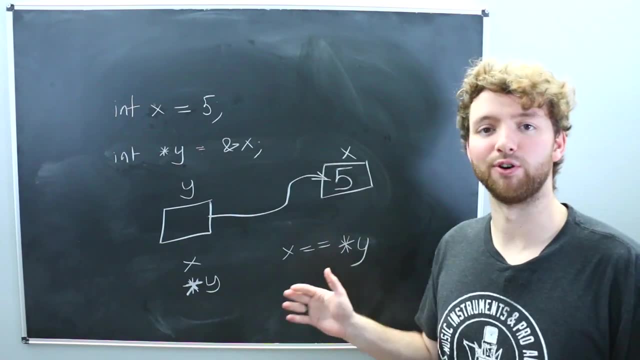 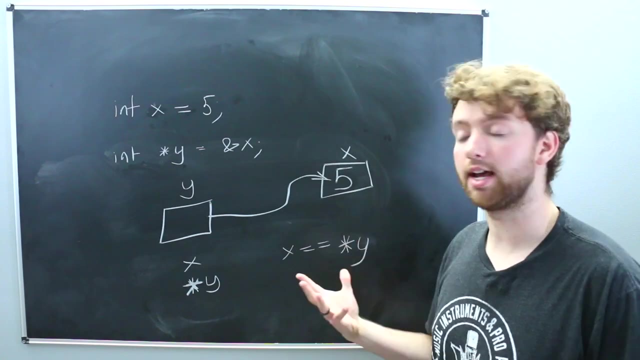 this should evaluate to true. Now I've been saying asterisk y, but that's not the official technical term of this. This is called the dereferencing operator. So we are dereferencing y to get the value that it points at. Now we're working with an integer, So just to. 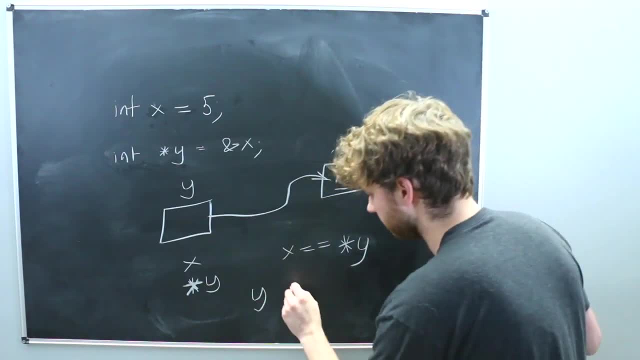 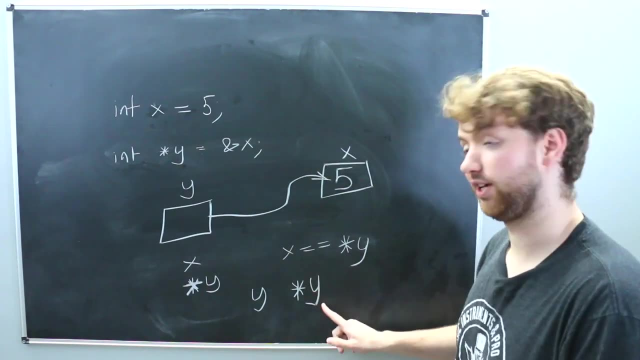 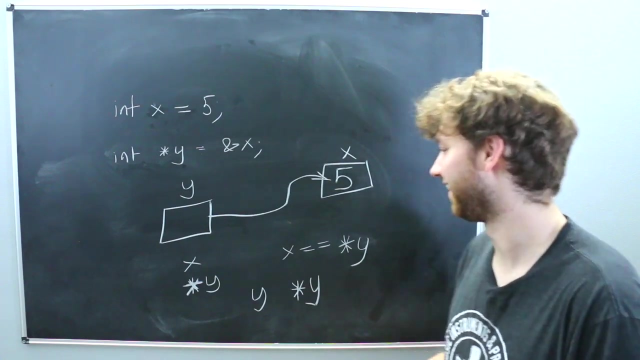 repeat that y is a pointer. Dereferencing y gives us an integer Integer, pointer, Integer, Integer, pointer, Integer. Say it with me guys. No, I'm not going to make you do that, All right. so this is where, like I, got the most confused when I first learned about pointer, I got the most confused. 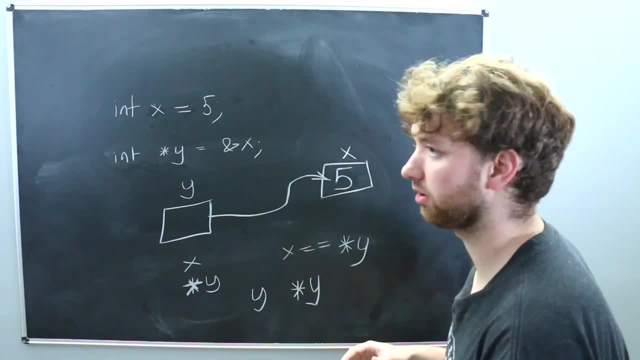 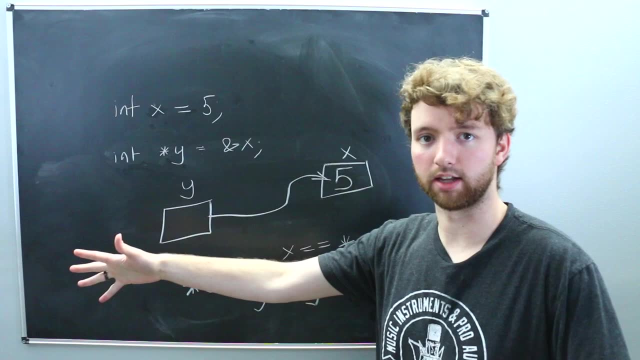 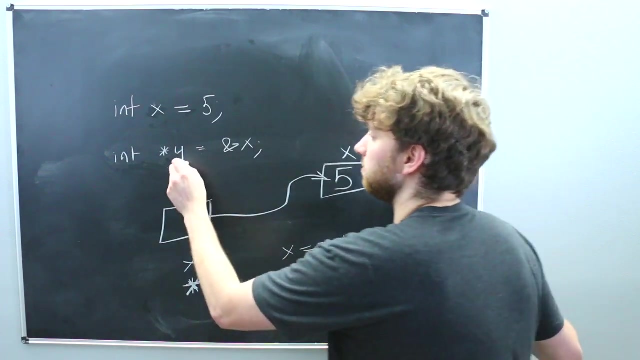 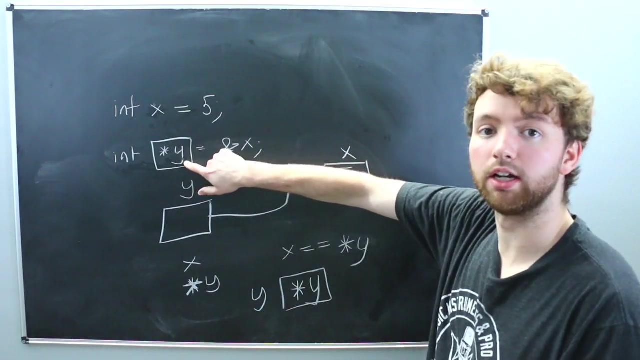 when I first learned about pointers and C programming. C programming, Disgusting. So you define the pointer using the asterisk. Okay, you got that so far. You can dereference the pointer using the asterisk, but these do not have the exact same meaning. This is saying: hey, we're creating a 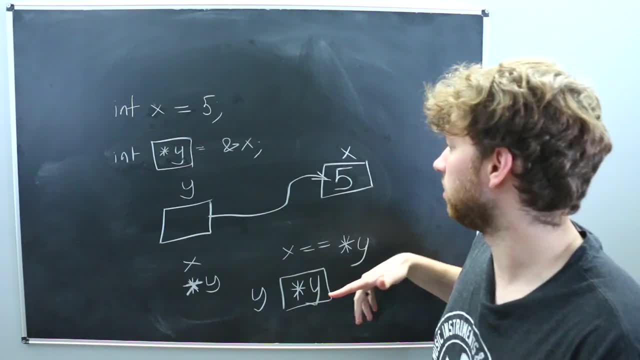 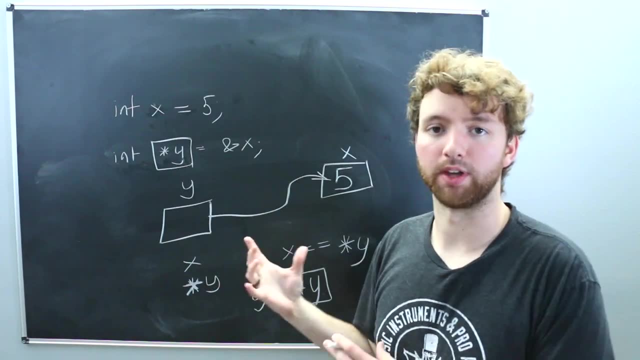 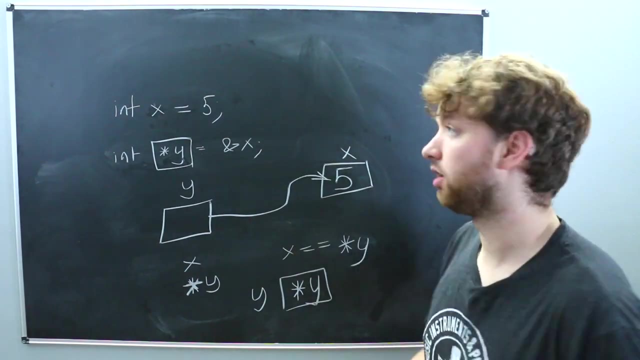 pointer. This is saying: hey, get the value wherever that pointer points. This is saying, hey, get the points to, but you don't have to use that asterisk whenever you're working with that pointer. you just use y by itself. so if i asked you, hey, could you write out the pointer you just created? you would. 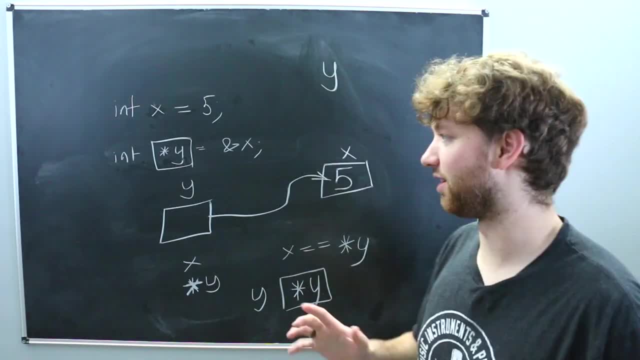 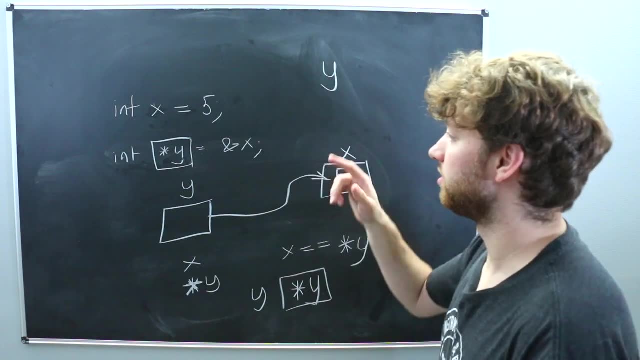 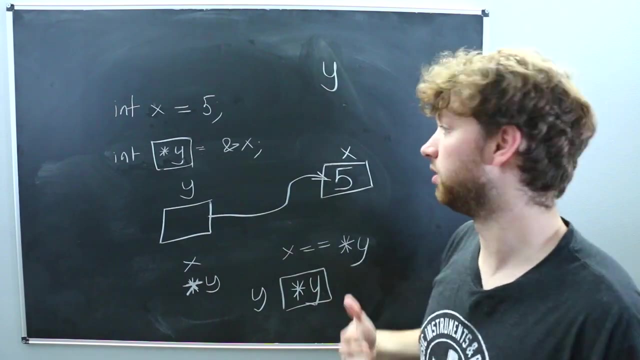 say y and it's confusing because when you define it you use the asterisk, but then you don't ever use the asterisk again until you want to dereference it. so asterisk to create the pointer. you use y by itself whenever you're talking about the pointer variable and then asterisk y. 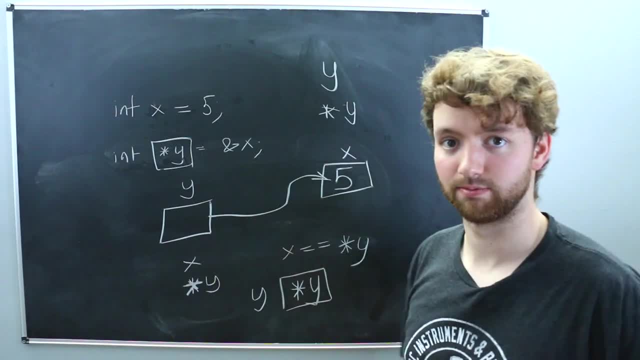 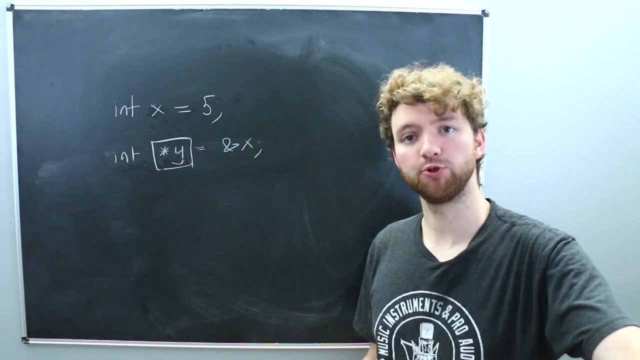 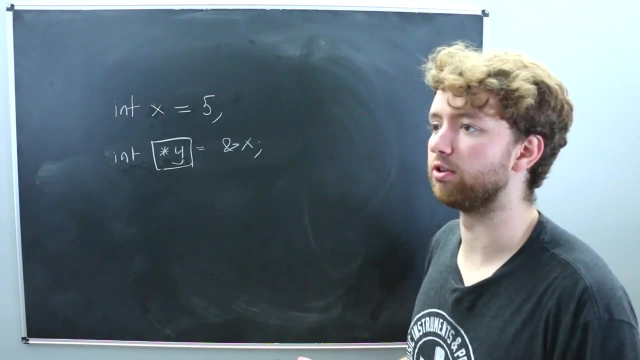 to get the data where the pointer points to. it's crazy, all right, why? why would you want to do any of this stuff? well, again, use references first, because you can do a lot of this stuff with references. however, let's just for a second. assume you had to use pointers. maybe you're using c. 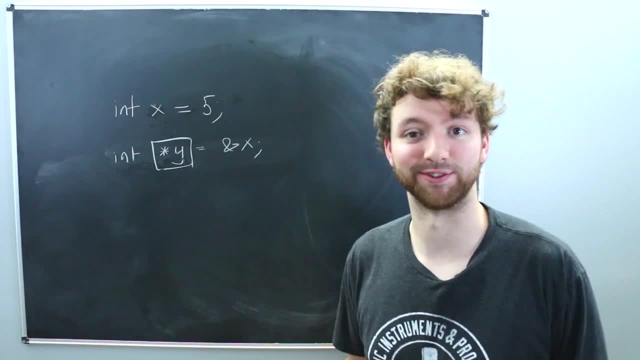 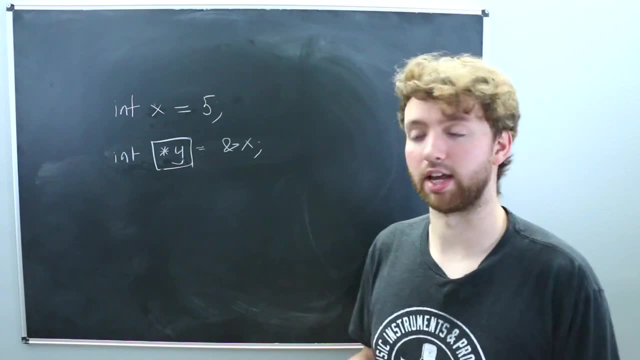 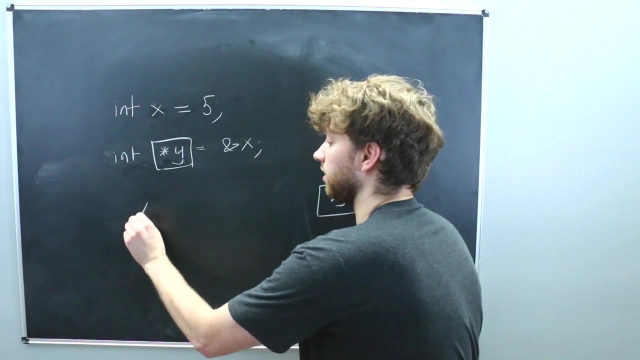 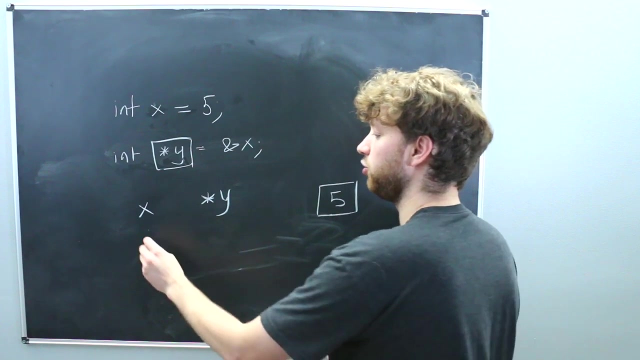 programming, or you're in school and they're making you use pointers for some reason. well, in that situation you can basically create two ways of working with the same data. to draw what i just had. this contained the value five, and you can refer to this data with x or by dereferencing the y pointer. so now you have two ways to refer. 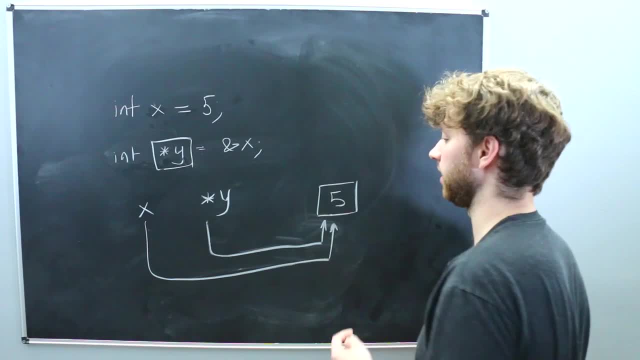 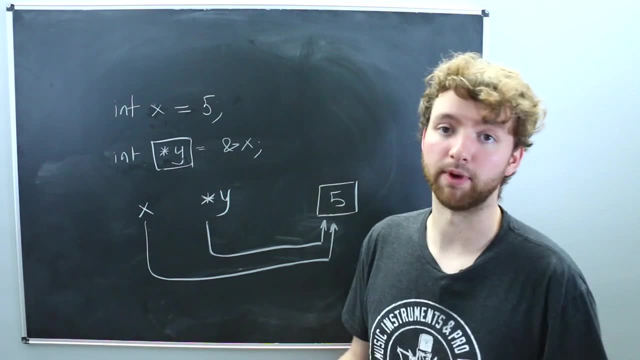 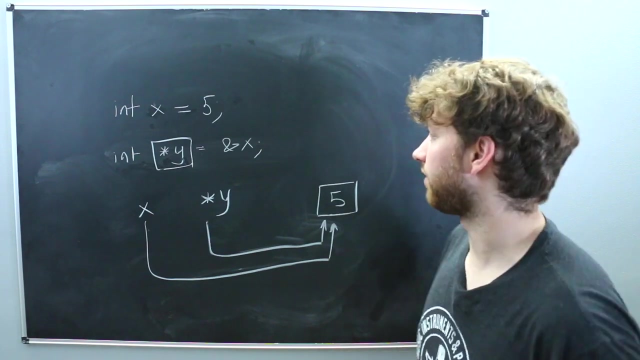 to the same location in memory. so that's the first reason you might want to do this. if you need multiple variables to talk about the same area of memory, you can use pointers. this is commonly used for functions and passing data. so if i create some function and you know it has a parameter in there, 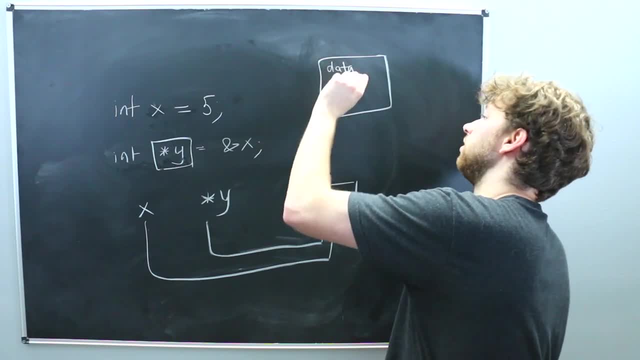 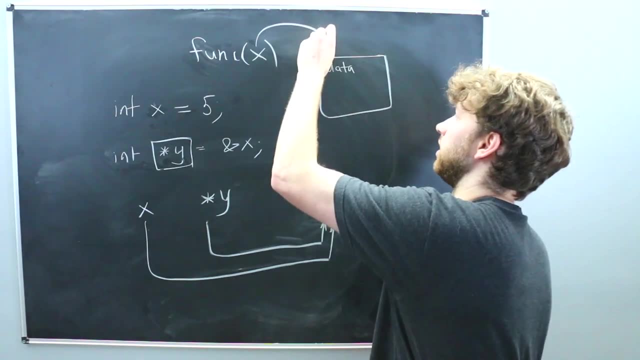 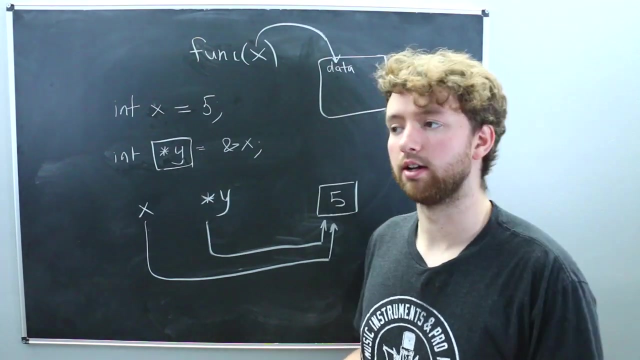 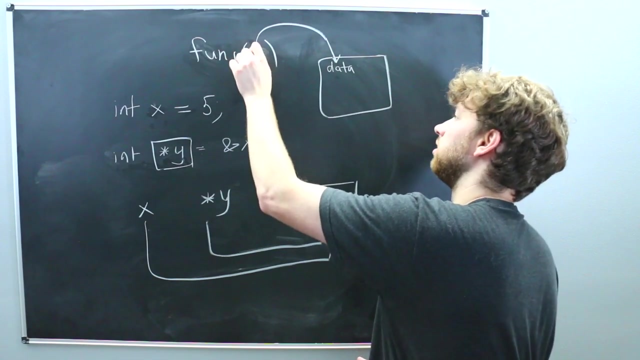 we'll just call it data. well, if you pass in x, by default that x gets copied. the data of x gets copied into this data parameter. well, if you're using pointers, you can actually have them refer to the same area of memory. so if, instead, you passed in y and the function took a pointer, well then, now the address is going. 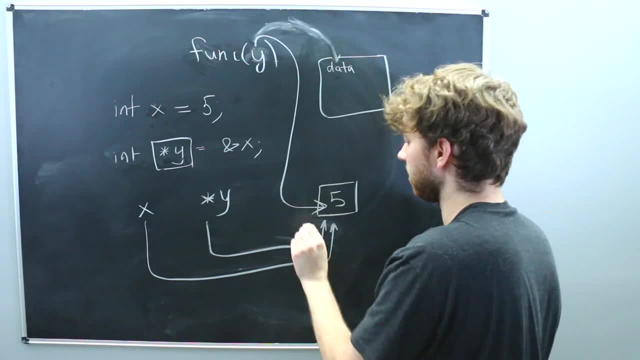 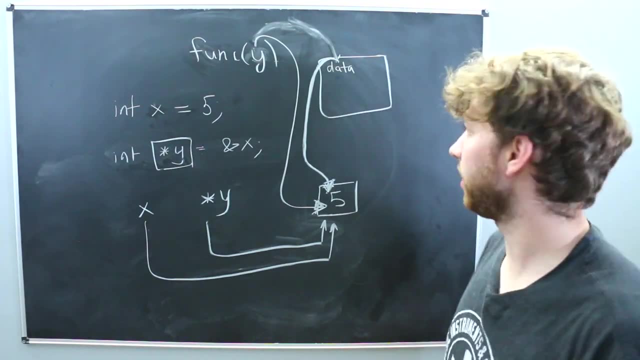 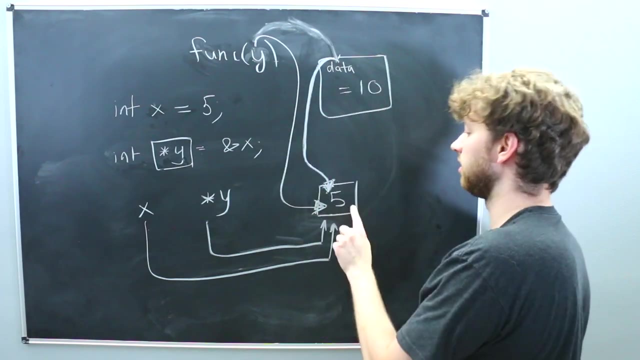 to be copied into data, and y is going to point to the same area of memory and data is going to point to the same area of memory. so what's the point now inside of this function? this function can change that data. So you know, we could assign it the value 10 and it's going to 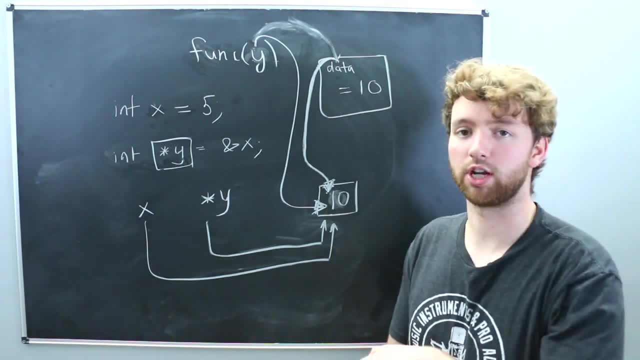 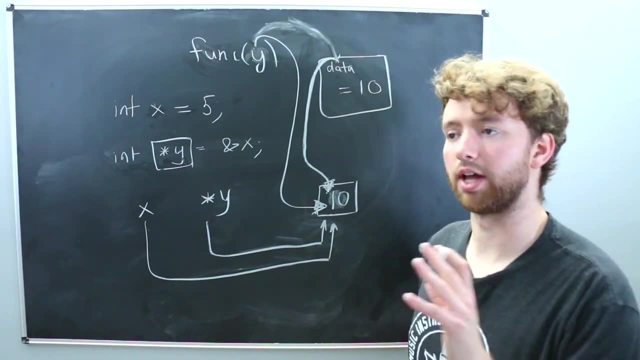 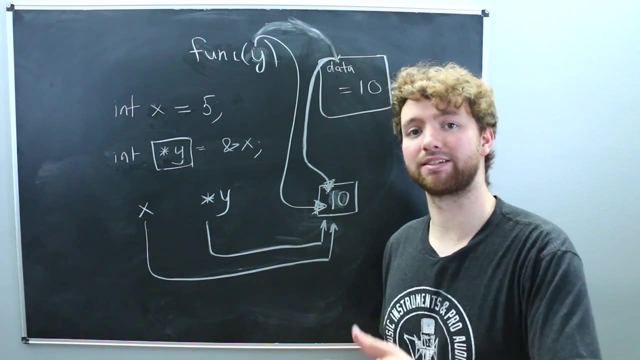 change that specific area of memory so that change is going to be seen everywhere, not just within that function. So, basically, we can use pointers to allow us to change data that's defined outside of the function. We can change the argument variables that are passed into the parameters and we'll see that. 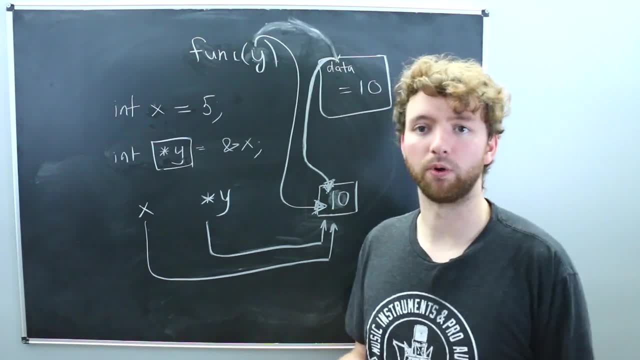 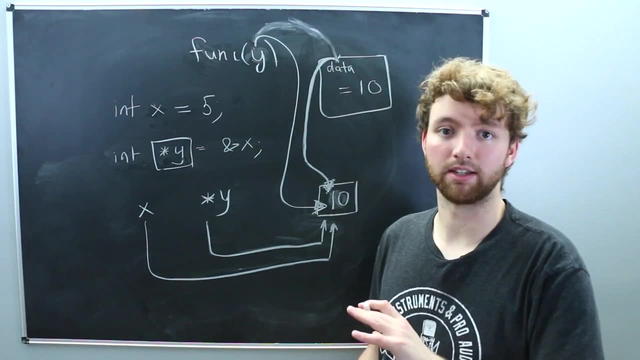 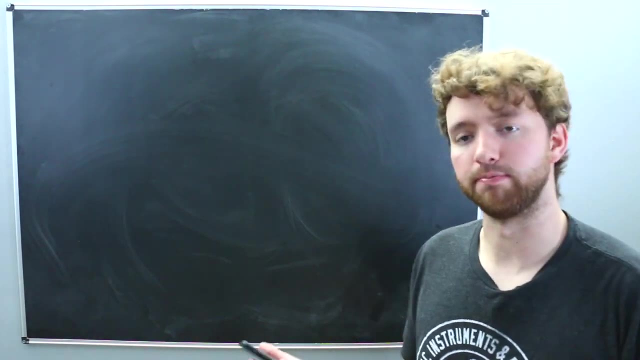 more hands-on in the upcoming videos. Don't worry about all the syntax right now. just understand the concept that it allows our functions to change data that's passed in and it's going to persist beyond that function call. You might see this for a swap function, so you could create a swap function to. 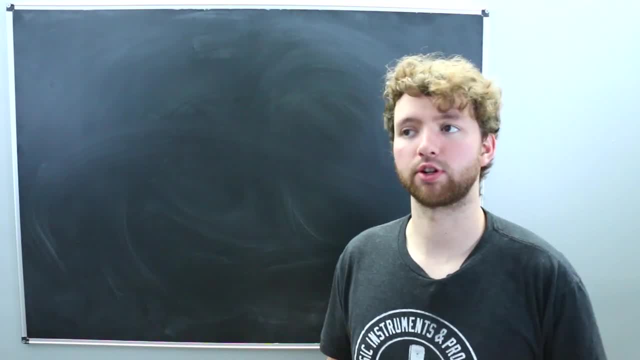 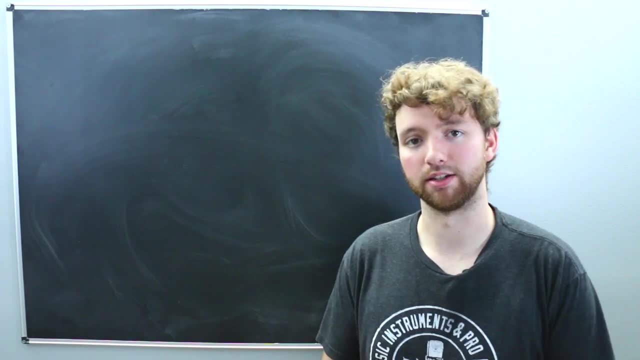 actually swap two variables. This is actually kind of hard to do in some other programming languages that don't have pointers or references, but in C++ it's really easy to do. You can do them with both pointers and references, because you can think of it like so: 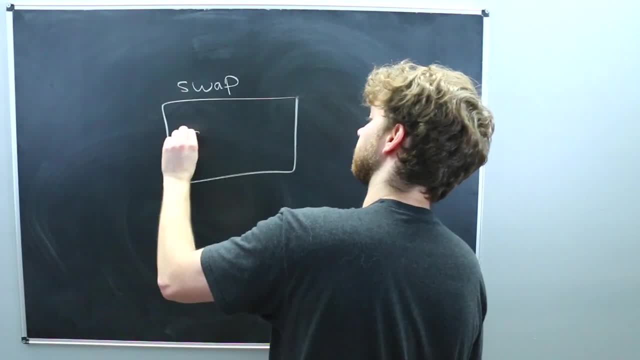 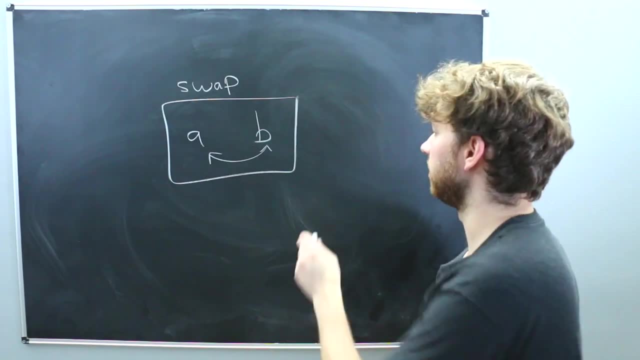 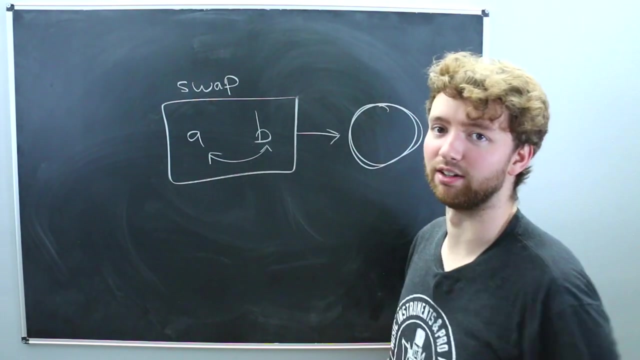 If we have some function swap and it takes an input A and input B and it swaps the data, well, in order for that change to be seen over here it kind of looks like a smiley face or like the Amazon logo- in order for those changes, 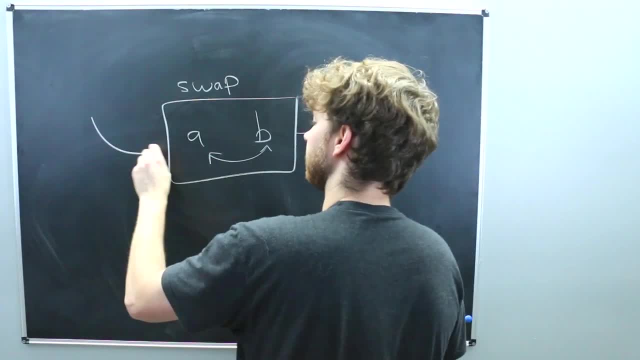 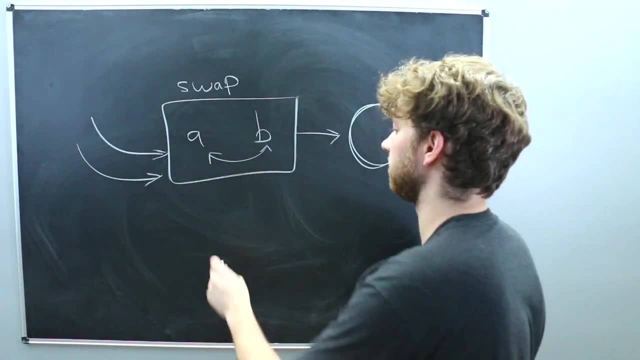 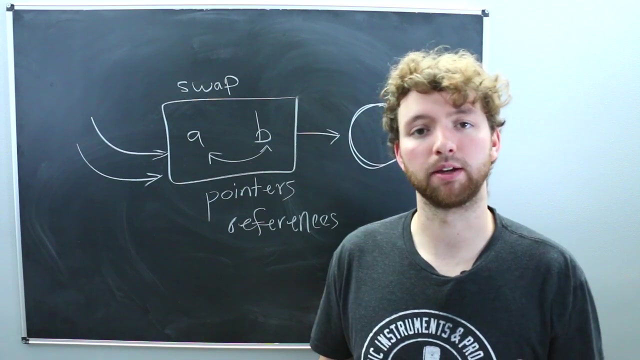 to be seen after the function call, that data that's passed in needs to be able to be changed, And again, that can be done with a function call. So in C++ you can do this with pointers and references, So any times you're. 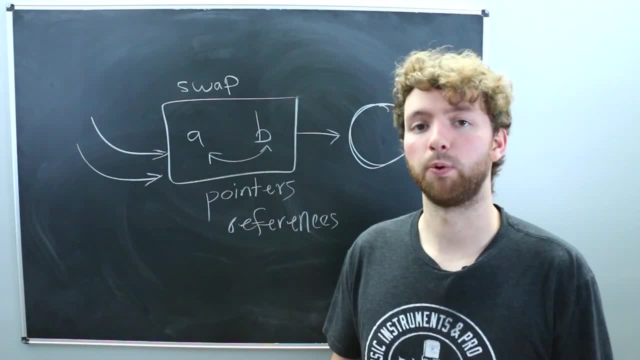 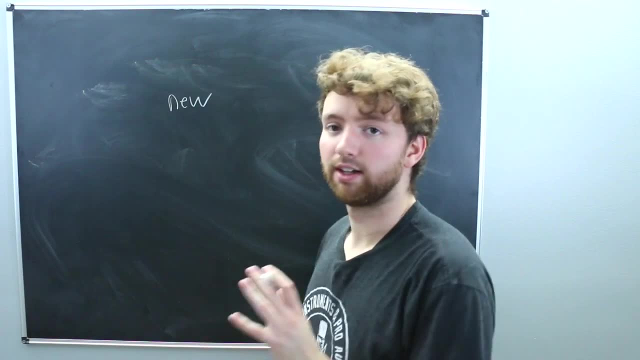 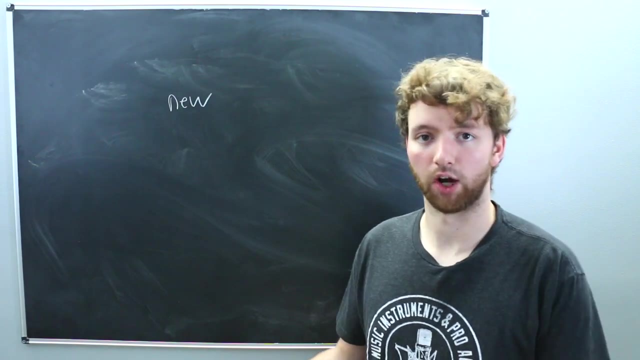 working with dynamic memory, where you have to allocate memory yourself, you're going to be using pointers. So in C++, when you see the new keyword that is dynamic memory allocation, and it's going to return a pointer, and you use that pointer to refer to that area of memory. 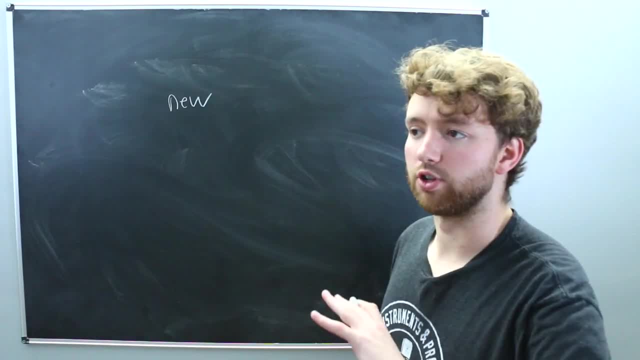 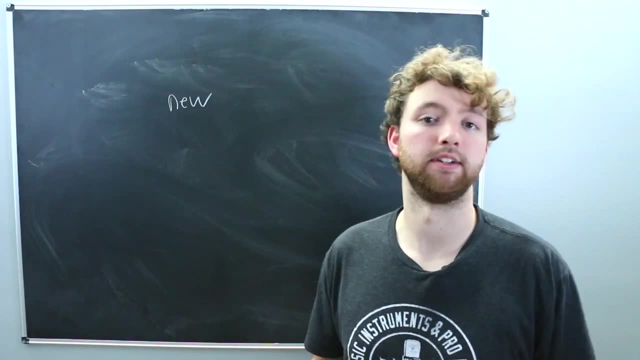 Don't do this unless you have to, and if you do have to, do dynamic memory. there's smart pointers which will kind of abstract away the memory management aspect of this. So you can study into smart pointers and the different types Inside of other programming languages. you know C-sharp, Java. you will see the 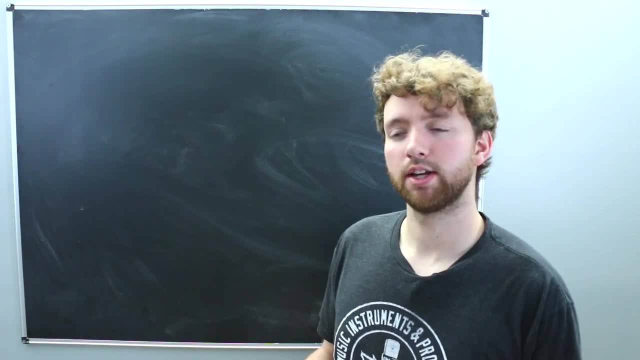 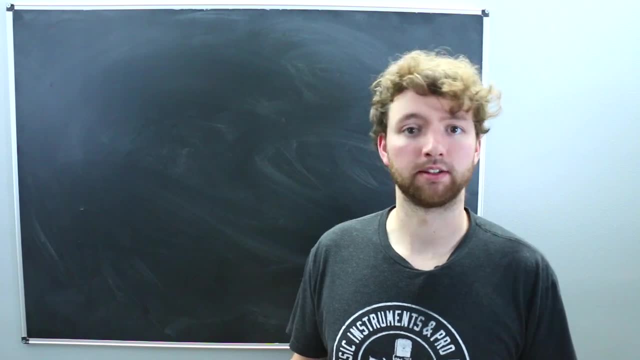 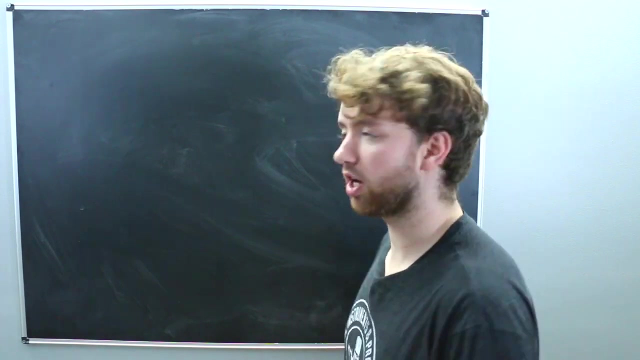 new keyword. quite often In C++ you don't want to use the new keyword unless you absolutely have to. In fact, when you create an object in C++, by default you don't want to use the new keyword. So if you're creating a user object, 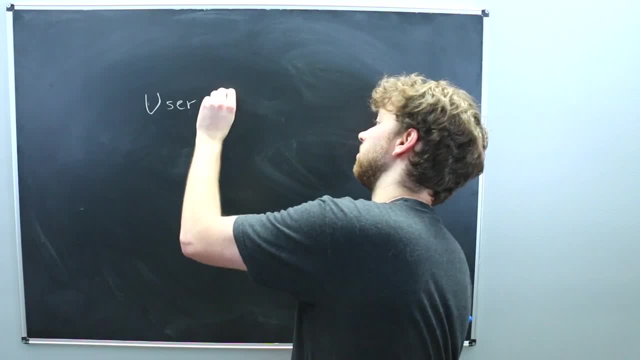 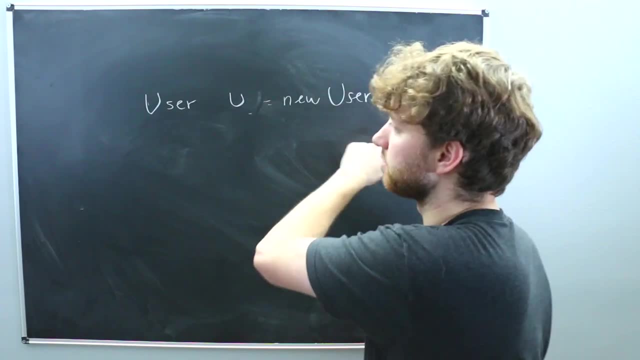 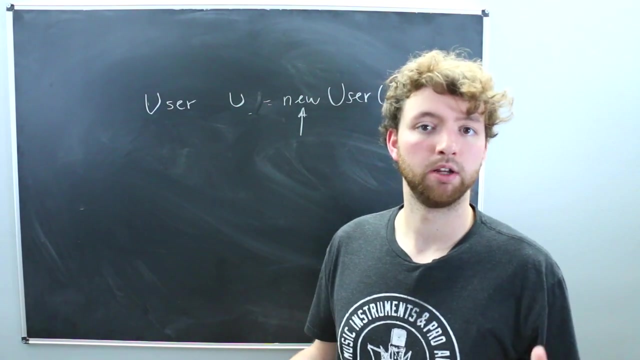 it's just gonna look like this: User U. you're not going to do something like this. This is what you would see in Java as an example, but in C++, this new keyword here is going to put this data on the heap memory and you're going to have to later. 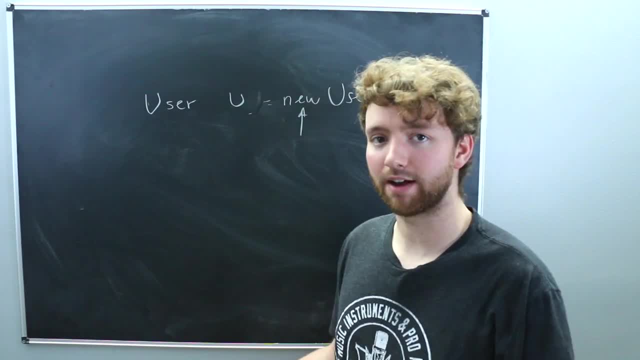 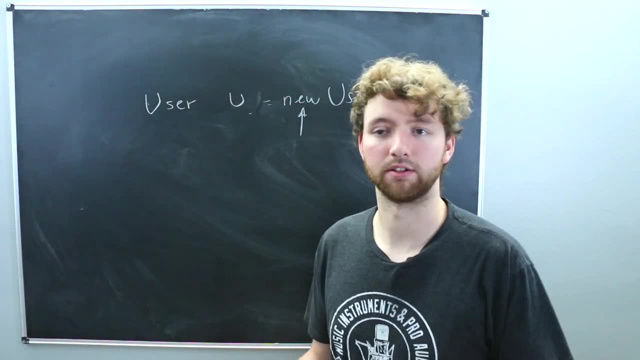 free this memory and you're gonna have to worry about that. So don't do that unless you absolutely have to for some reason, such as if you need this to extend beyond the scope it's defined in. But we're really getting into the weeds here. 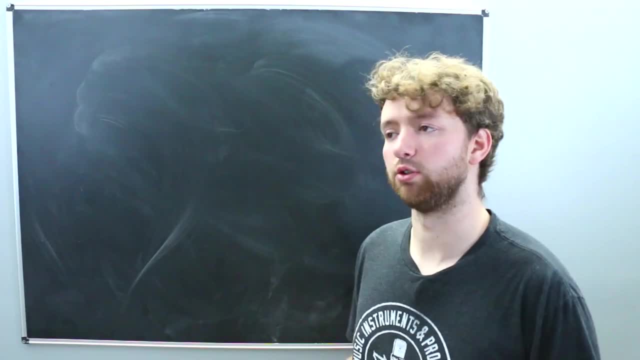 so let's not worry about that right now. So I think that's going to conclude my introduction to pointers. Check out the next video because we're going to get hands on with it And if you're looking for a little bit of extra study, 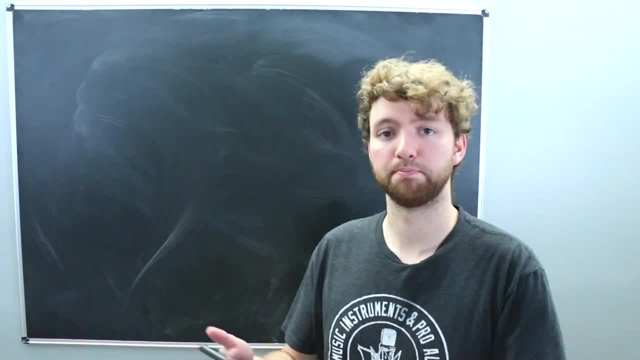 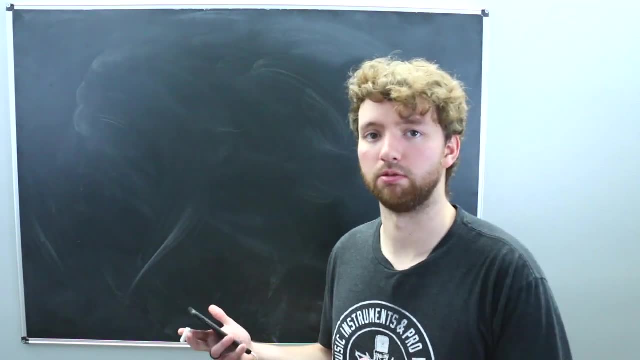 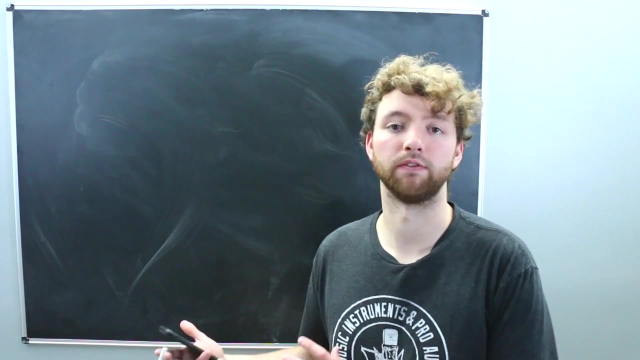 I suggest you look up differences between references and pointers. So we talked about references, we talked about pointers. now you just need to figure out when you want to use which. And again, just to repeat myself like the fifth time: use references unless you absolutely have to use a pointer for something. 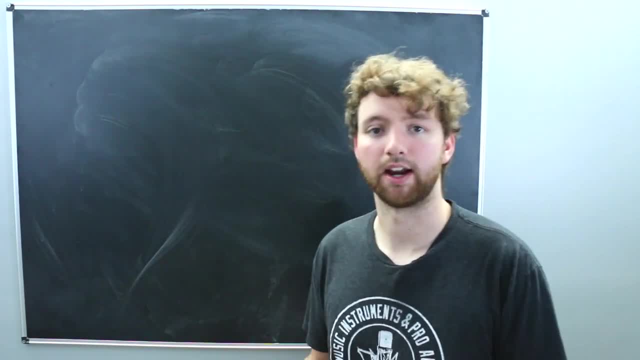 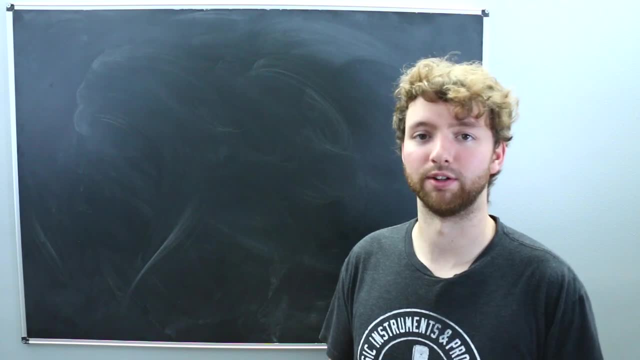 But most of the time that's not going to be necessary. For example, I did a 10 hour C++ series here on YouTube and everyone was so upset because I didn't get into pointers. It's because I had absolutely no need for the pointers.